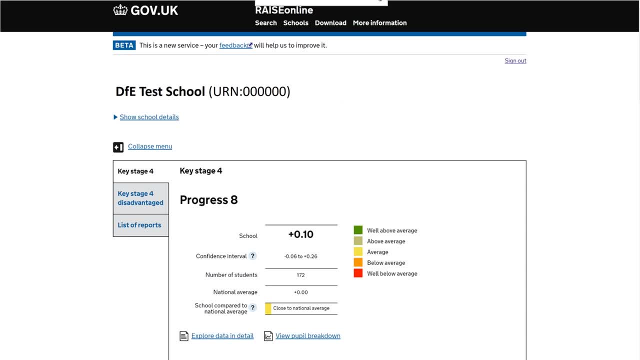 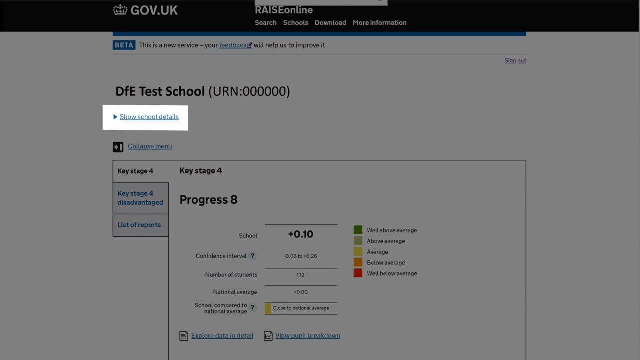 So simply enter your username and password and you can log on. Once you've logged on, it will take you to the learning page of your school. Here you can see a summary view of your school details by clicking on the drop down arrow provided. 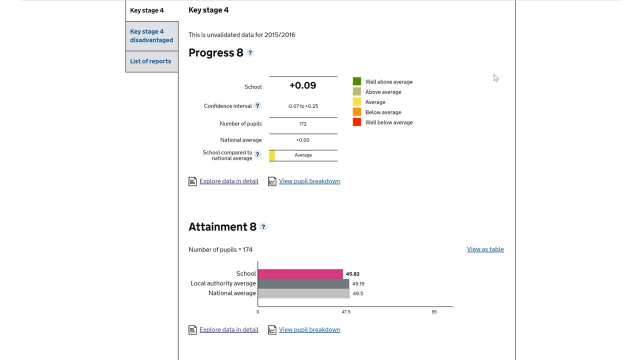 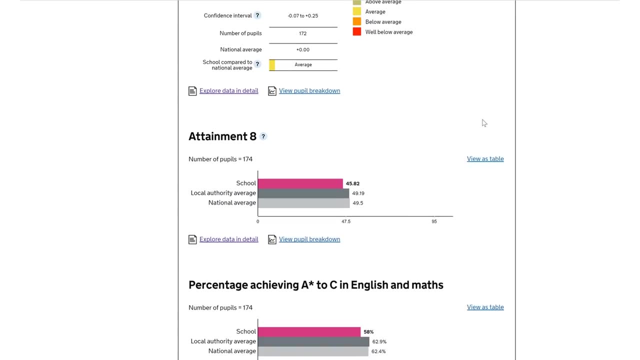 Ok, so let's have a look at the performance headline information. You can see that this is all on the same page. Simply scroll down to see the different measures. Starting with Progress 8, we go to Attainment 8, Percentage achieving A star, to C in English. 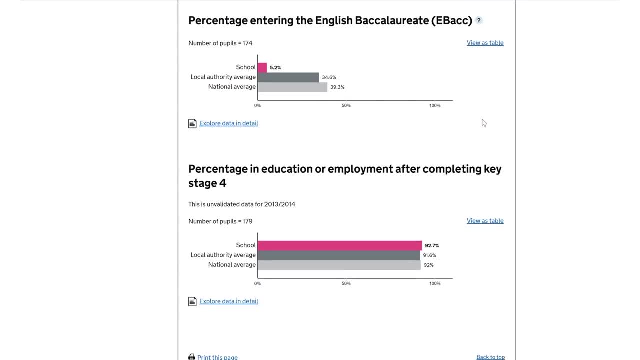 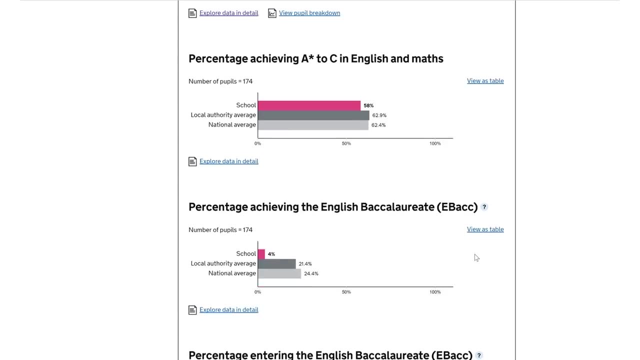 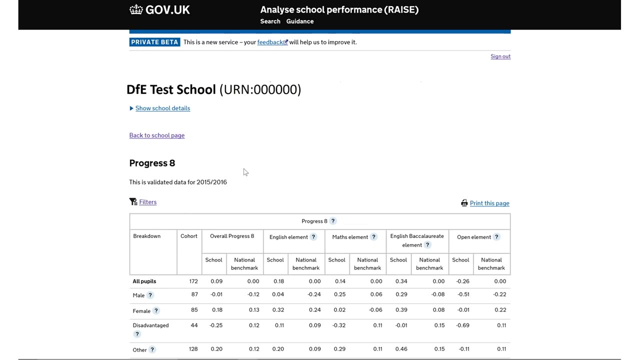 and Maths. Then we have English Baccalaureate, Entering the EBAC, and finally, the Destinations measure. We also give you the option to view as a bar chart or as a table. Each measure also has the option to view the data in more detail. This provides a more 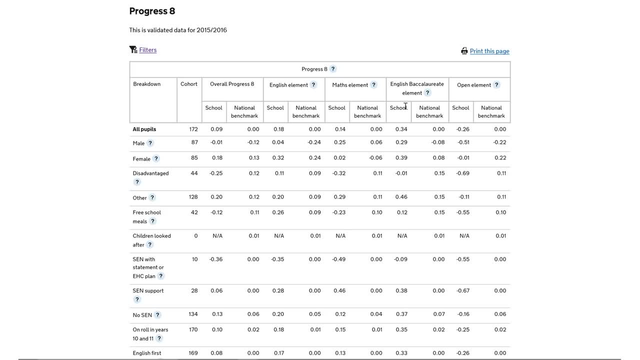 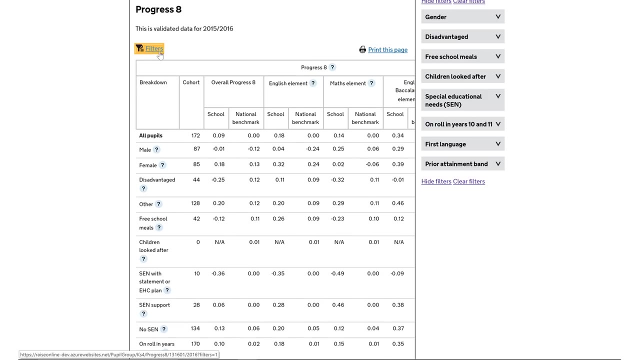 detailed breakdown of performance across the measure. So, for example, with Progress 8, we can see all the different elements and the breakdown by key pupil groups, such as Gender, Disadvantaged, SEN, etc. You can also filter this by clicking here and opening up the filters. So let's say we 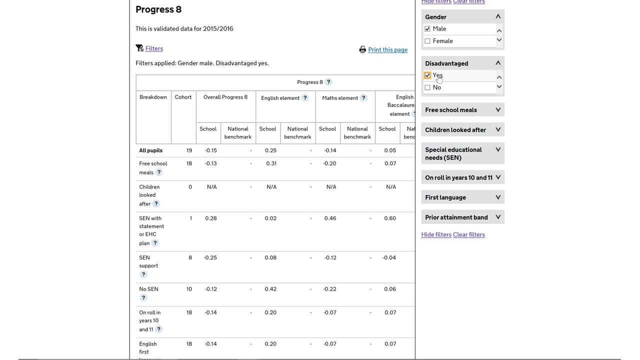 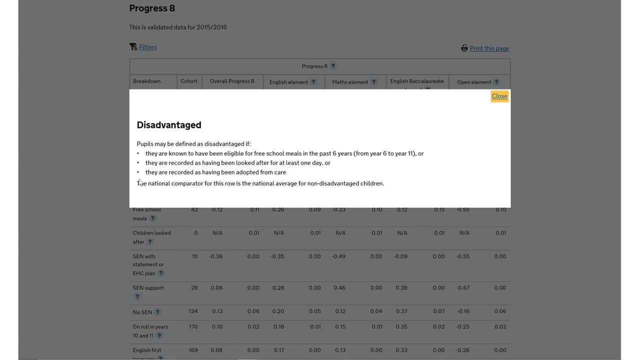 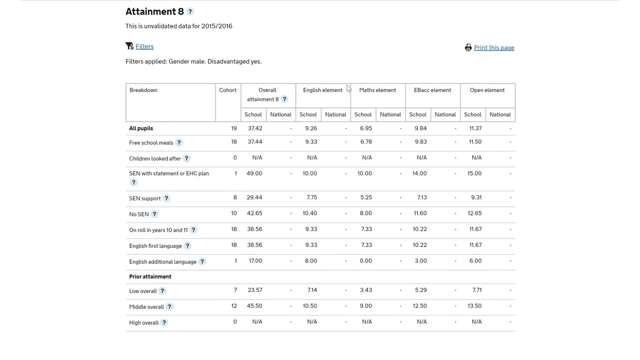 want to look at how disadvantaged boys are doing, we simply click on Disadvantaged and Boys Within the tables. there is also the opportunity to remind yourself what the definitions refer to by clicking on the question marks. Finally, there is also the ability to print the reports or save to PDF. 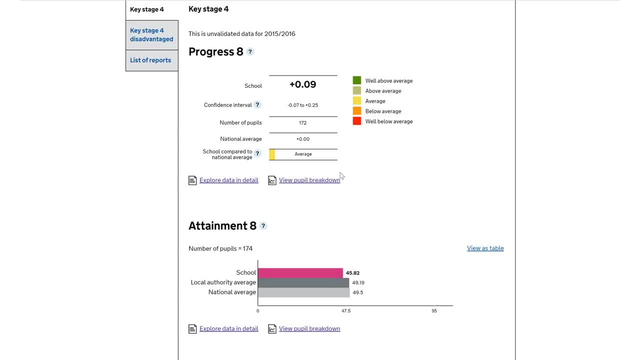 Ok, so let's go back to the front page. Let's now look at the report that we just created. We can see that we have a list of all the data we want to view. We can also see that we have a list of all the data that we want to view. We can also see that we have a list. 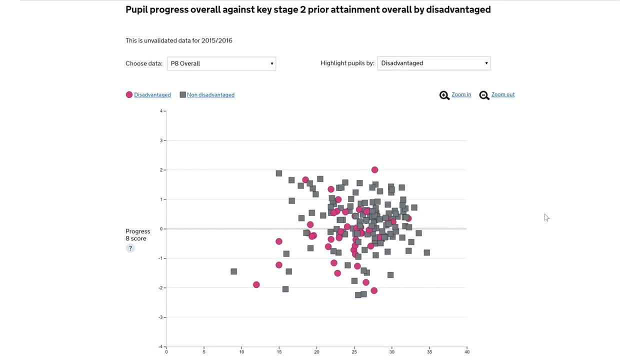 of all the data we want to view. We can also see that we have a list of all the data that we want to view, So let's now import that list and reflections here. These scatter plots enable you to easily see if there are any patterns of performance. 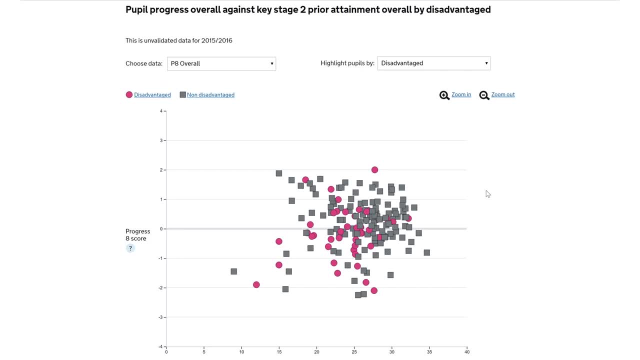 in your school and to easily identify outliers. So, for example, let's say, the majority of the pupils at this school are performing above-average, but there are few who are significantly below. Why is that? Here you can look into the details of each pupil by clicking on the dot. You also have 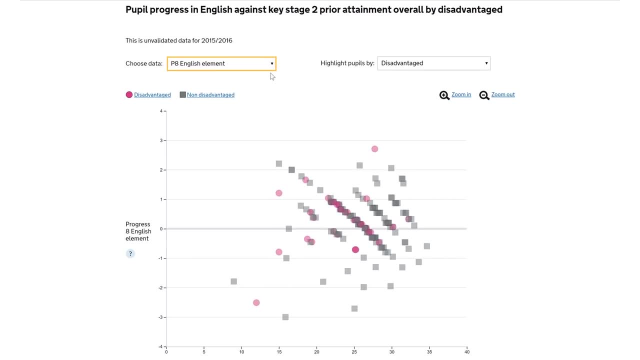 the options to choose the data for each subject and to highlight different pupil groups. We know that this functionality has been very well received by governors, who are keen to see if their school development plan and priorities are reflected in the outcomes. For example, if they have been investing in maths, are they seeing the results that they were expecting?